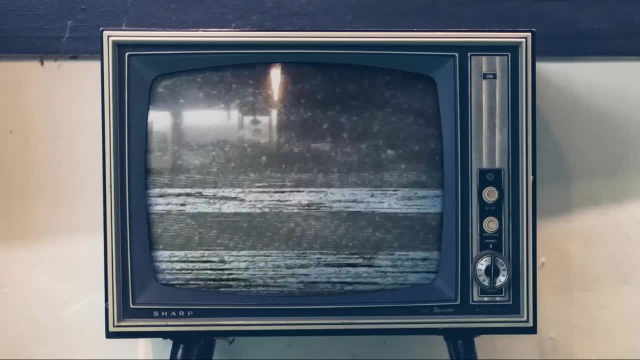 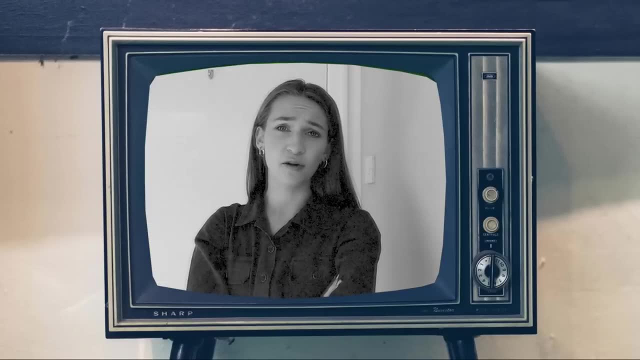 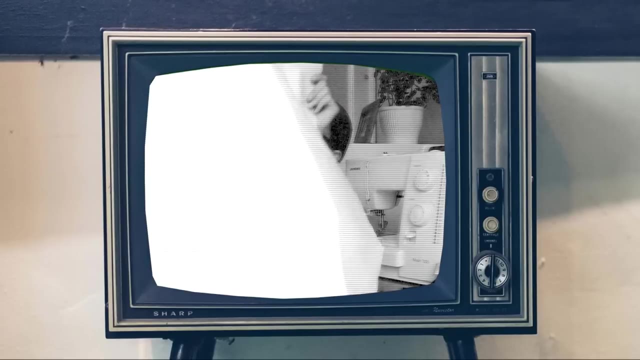 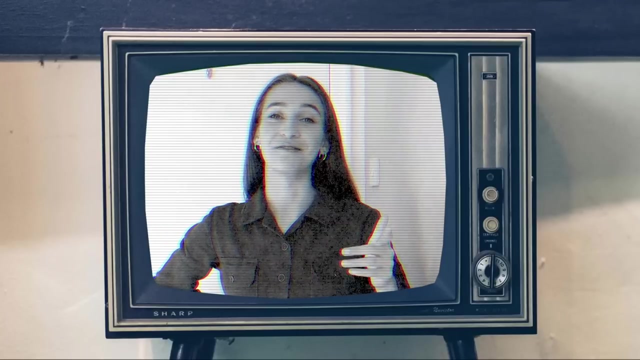 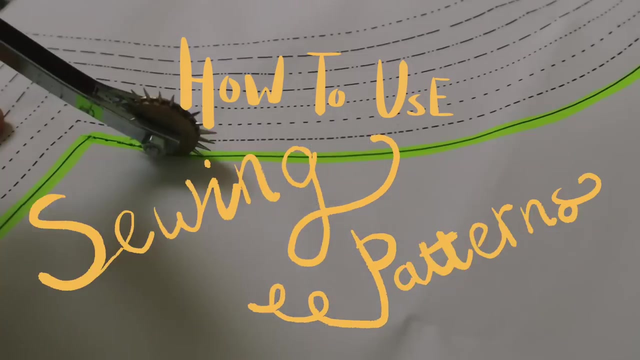 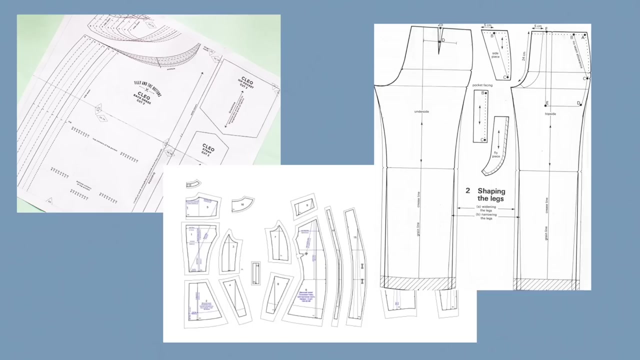 Would you like to learn how to make your own clothes? Yes, Do you find yourself lost and bewildered at the mere sight of a sewing pattern? If that is you, then welcome. You have clicked on the right video. This is a sewing pattern. It looks confusing at first and 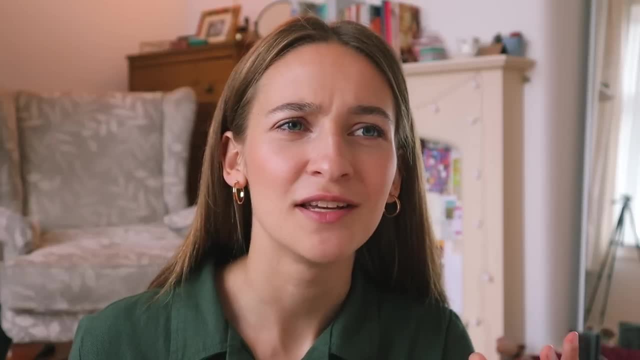 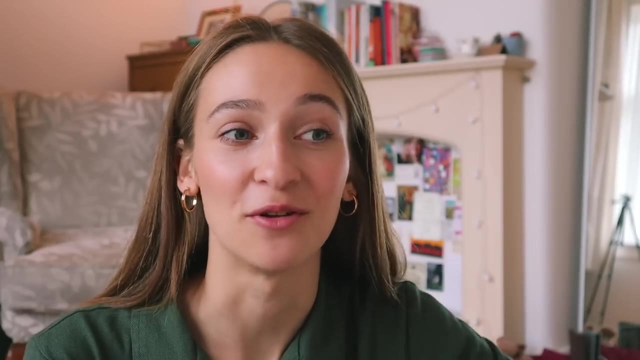 intimidating and just kind of weird. I mean, how do these random contorted shapes turn into something that you can actually wear? If you would like to know the basics of how to read and understand and make your own clothes, then please do so If you have any questions. 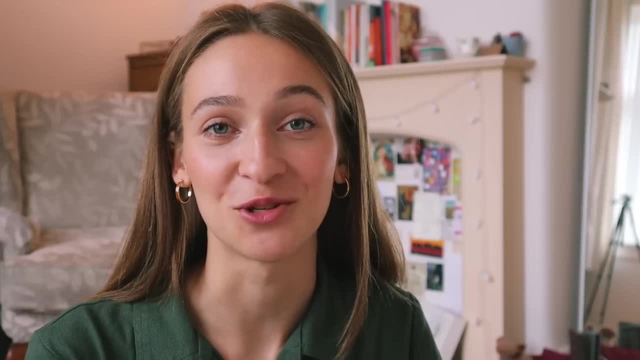 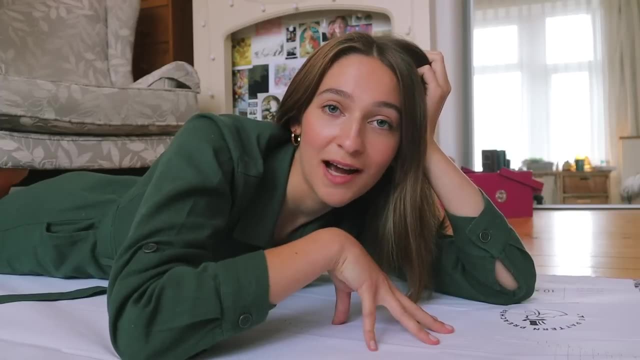 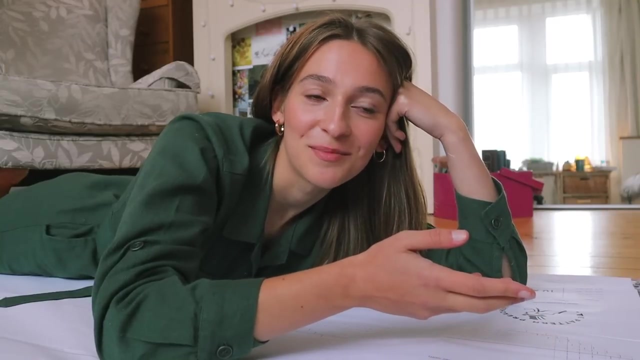 please keep on watching because I'm going to show you how I used a pattern to make these palazzo pants. Okay, sewing patterns come in a range of different sizes, obviously, since we all come in different shapes and sizes And the different sizes are usually represented. 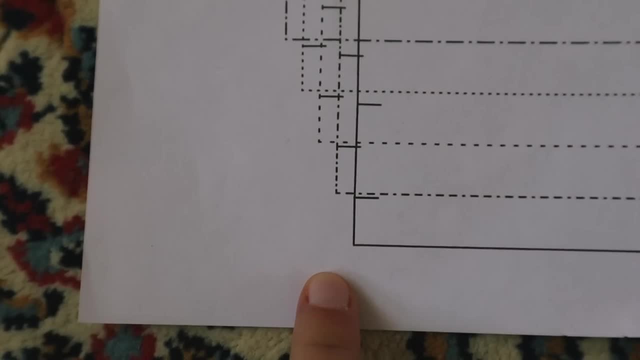 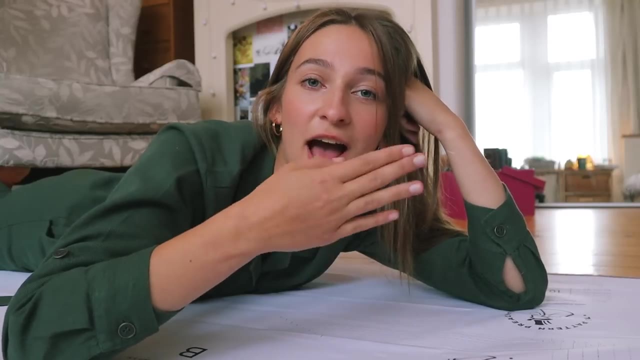 by different styles of lines so that you can easily distinguish between them. So you can go right ahead, find your size and cut it out for yourself. If you have any questions, please let me know. If you have any questions, please feel free to leave a comment below So I'll. 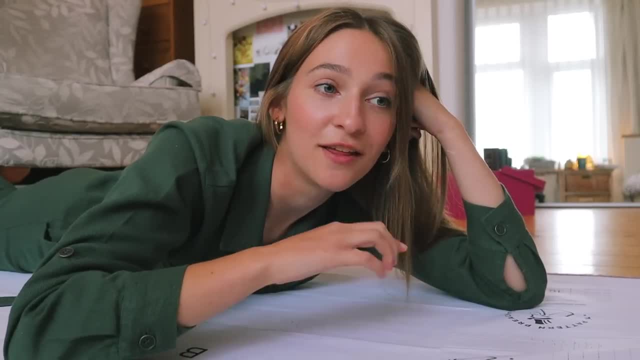 see you in the next video and I'll see you then. You may have noticed that I cut it straight from the pattern. However, if you do this, you are not taking full advantage of your sewing pattern. Once you cut directly into the pattern, there is no going back and you no longer have access to any of the other. 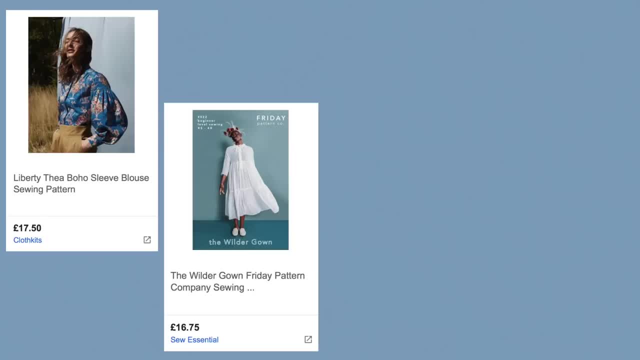 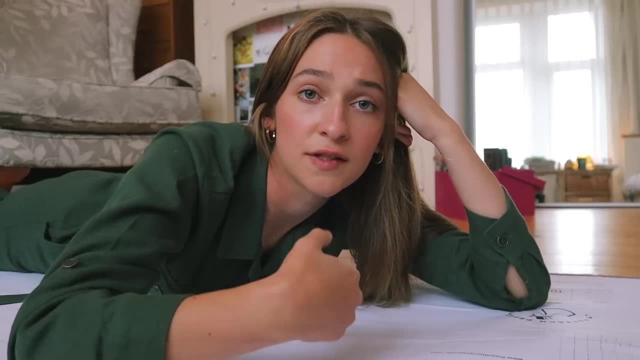 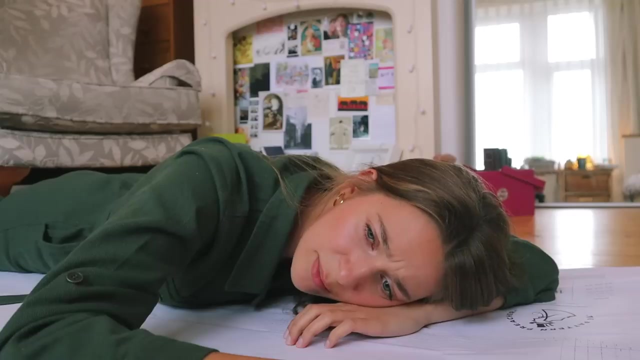 sizes that the pattern has to offer. Also, patterns can be kind of pricey, So you do have to think about value for money. And you might want to make this for someone else who's a different size- change size, I mean, it happens- and then you might think, damn it, I don't fit my. 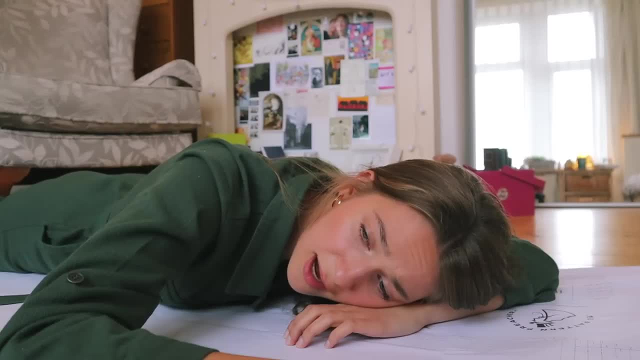 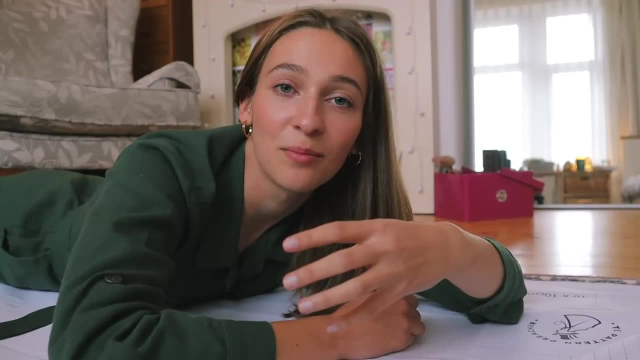 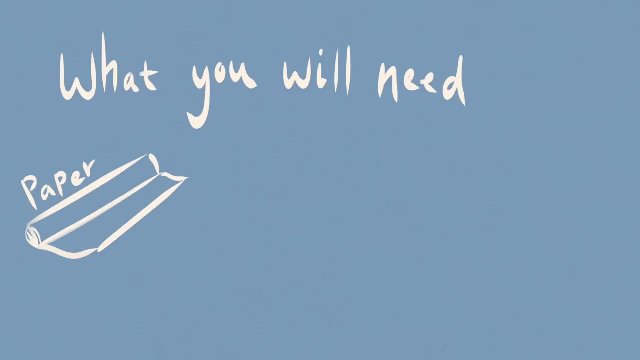 palazzo pants anymore. I wish I still had my full pattern with all the sizes still there. instead, the most efficient way is to trace the pattern, and that means you are not wasting anything. for tracing you will need some paper, a ruler, scissors, marker, highlighter, tracing wheel and an awl- and those last two things which also 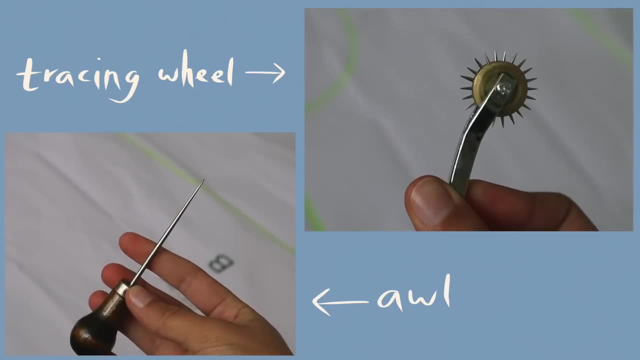 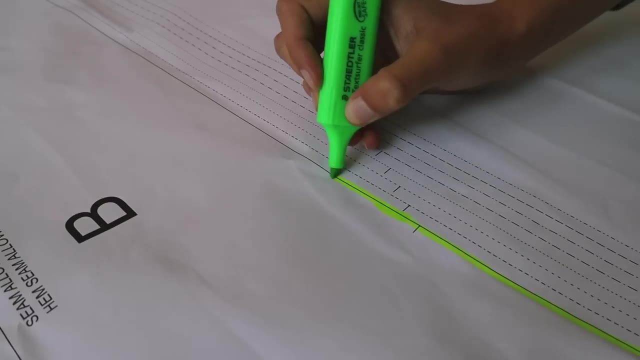 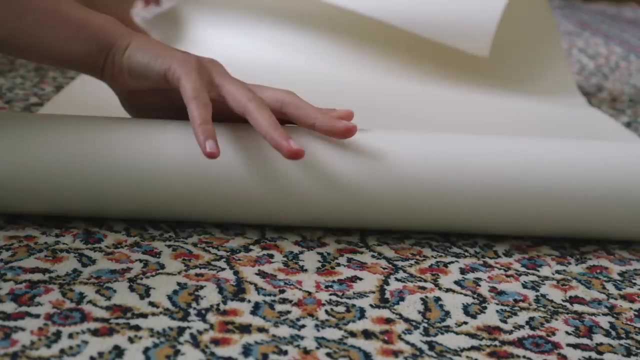 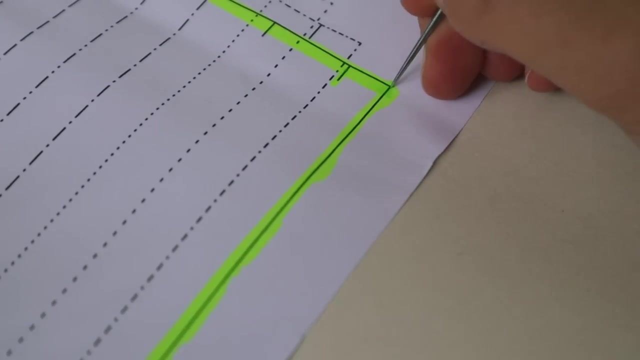 look like they could be. torture devices are optional and if you don't have them, you can improvise by using regular pins. okay, so we start by finding our size and highlighting the corresponding lines. roll out your paper and lay your pattern flat on top, grab your awl or basically any other poking device and pierce. 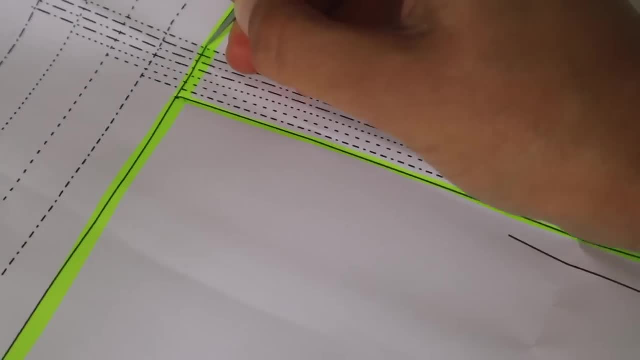 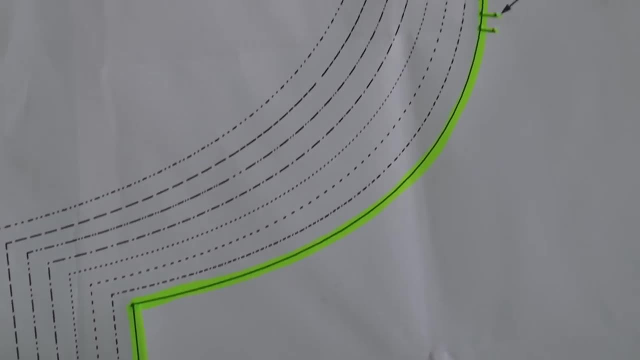 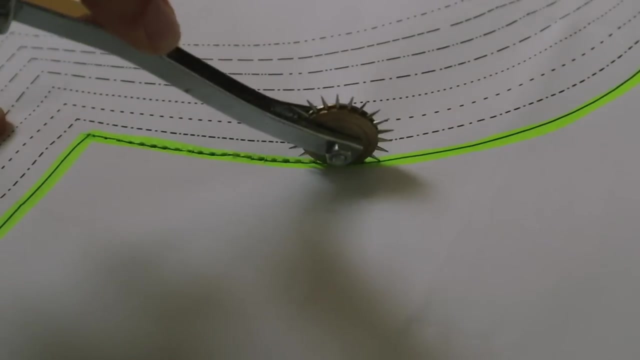 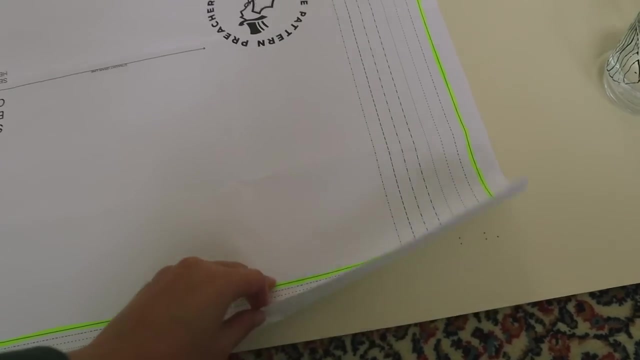 the darts, etc. and to mark lines on your pattern that are not straight but instead are curved. grab your tracing wheel and follow the curve with it, and, if you're using a pin instead, simply pierce lots of holes along the curve for the same effect. and once you have finished with your piercing, it's time to 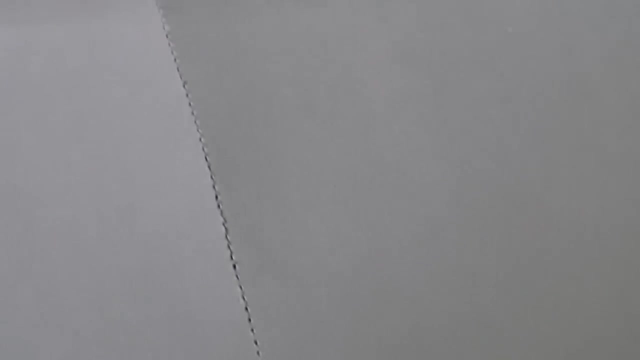 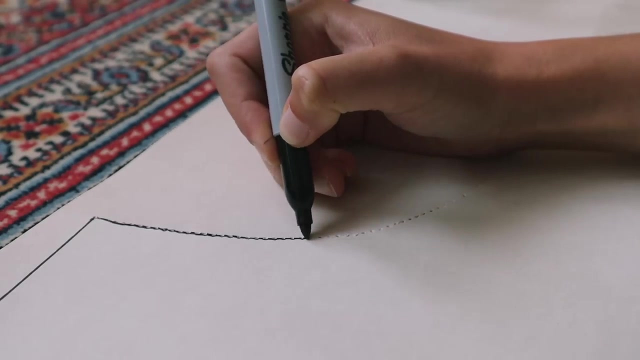 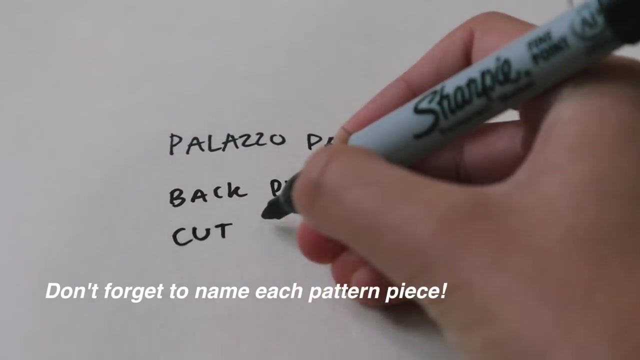 remove the pattern and basically join the dots. so grab your ruler and your marker and go ahead adding in the straight lines, the curved lines and any markings that the piece has, like notches, darts, grain line, etc. your piece should now be complete and ready to cut out. and once you've done this, with all of 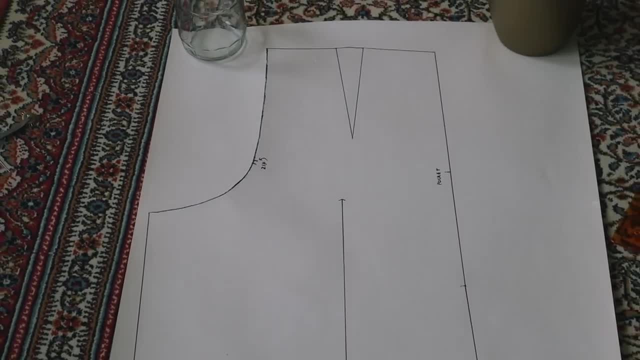 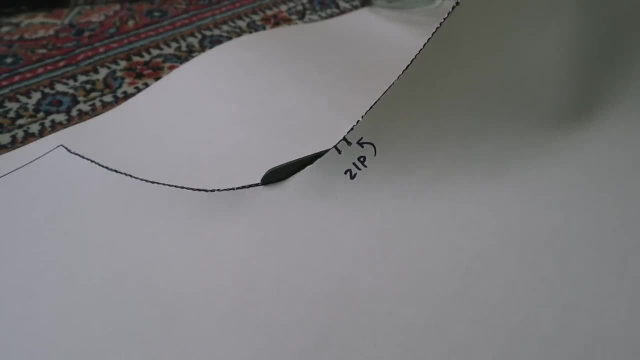 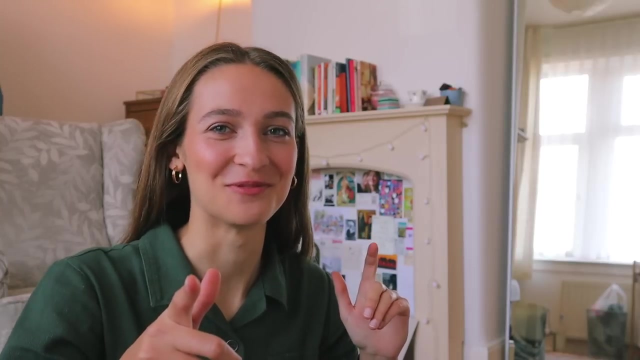 the pattern pieces. you are ready to move on to the next stage, but first, as this as a video for beginners, let's talk about the symbols and what they actually mean. let's talk about symbols and not the percussion instrument. symbols are part of what makes sewing patterns so intimidating. I think because 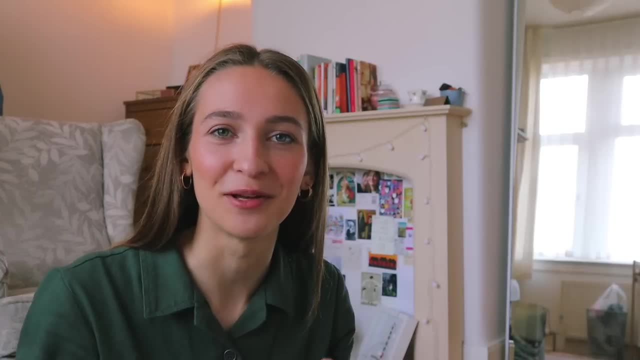 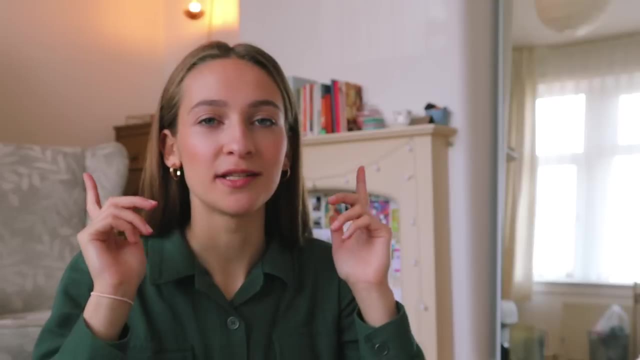 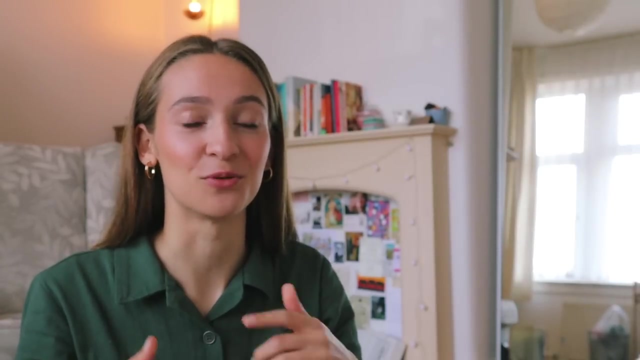 it's all these weird ass shapes just peppered around every pattern piece and you have to somehow know what they all mean in a practical sewing sense. but once you know them, you know them and they're actually pretty easy to follow. the symbols are essentially there to make the sewing process easier, so they're. 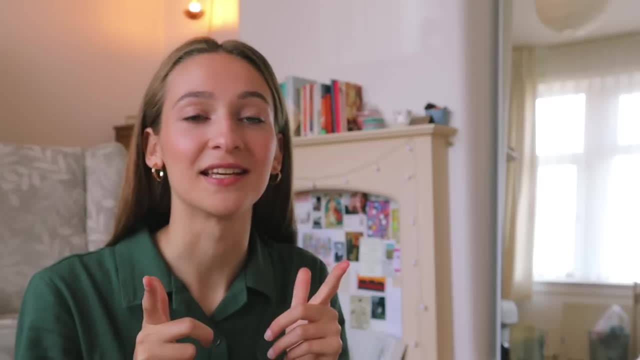 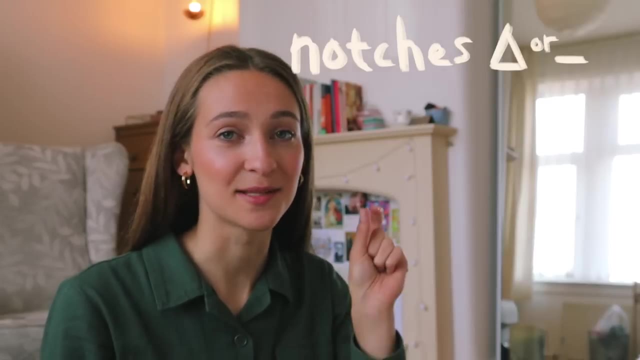 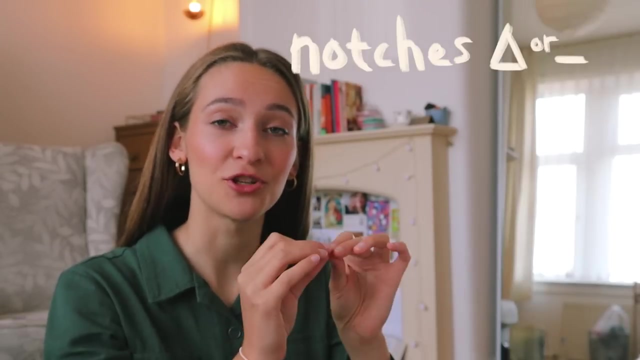 good. so here is a run-through of the most common and basic symbols. number one: most common symbol: notches. notches are usually marked by small lines or small triangles at the edge of a pattern piece. these are essentially guides for you to be able to match your pattern pieces at the right spots. they're actually really. 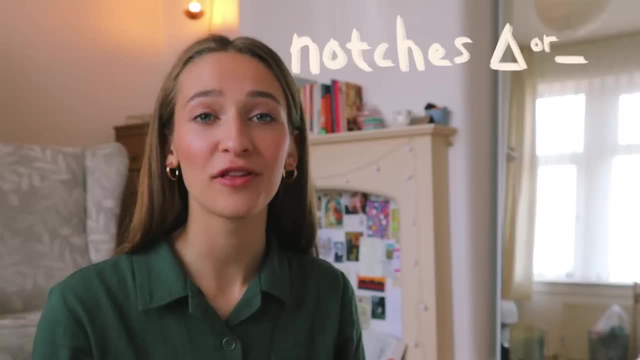 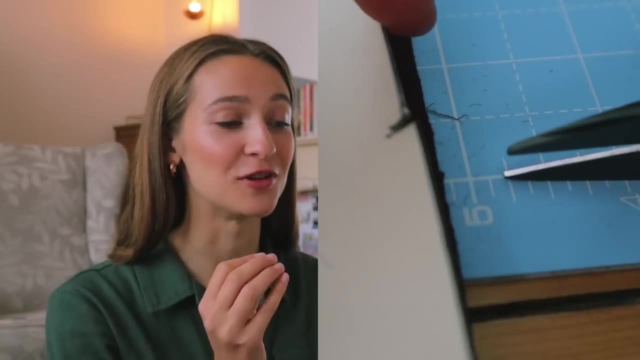 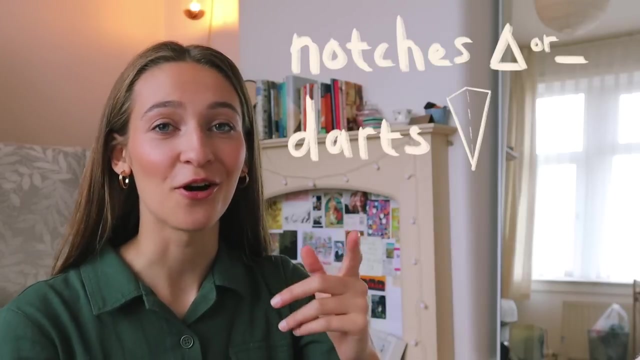 important if you want your work to be accurate and neat, and all the symbol is asking you to do is snip a little bit of the fabric where the notch is, and you have a visual guide for where you need to match your pattern pieces. the next is darts- And no, not the boring game that old men watch in pubs. I'm sorry these. 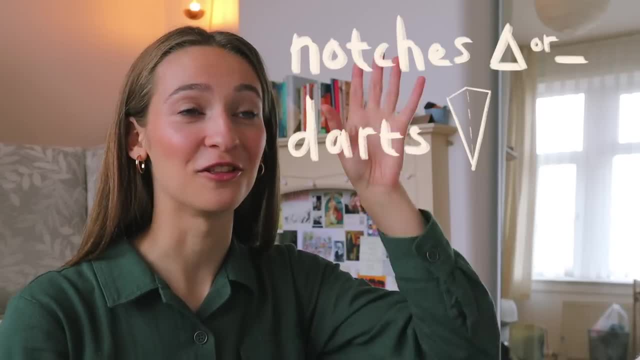 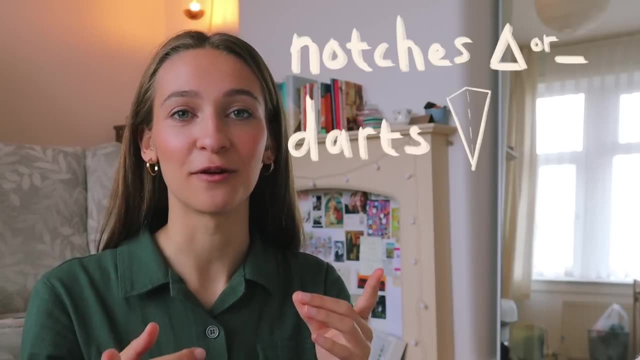 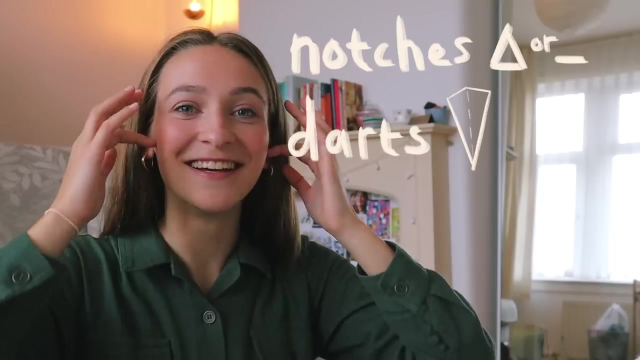 jokes are terrible, And these are represented by larger triangles. Darts are crucial for adding body and shape into a garment. Typically, they're found at the bust and at the waist, you know, because those are typically the places that your body has curves. All you need to do is mark these accurately on. 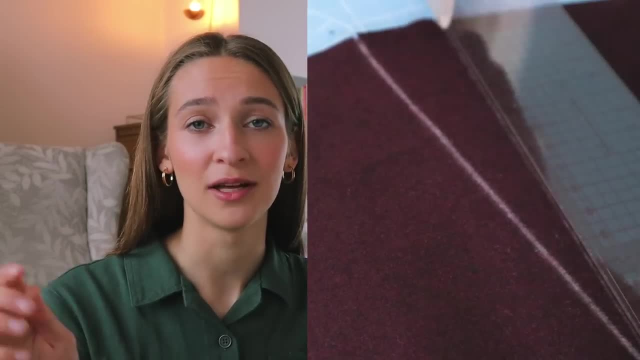 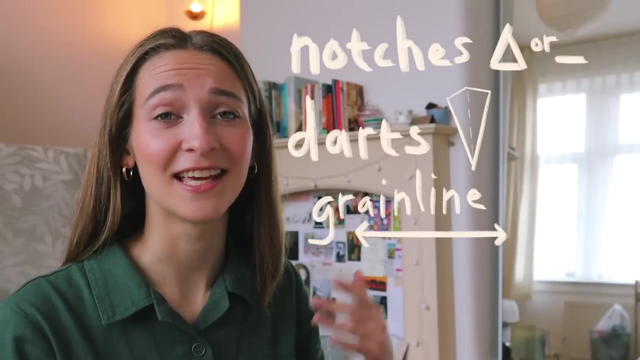 to your fabric, either with some chalk or a pencil, and then you can see clearly where they are before you sew them in. Next we have the grain line, and this is just a huge, big arrow across the center of your pattern piece. The grain line. 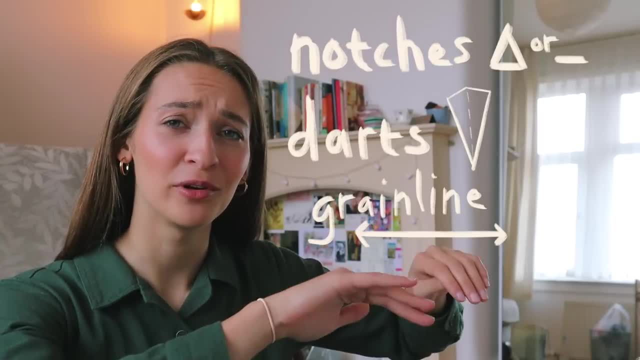 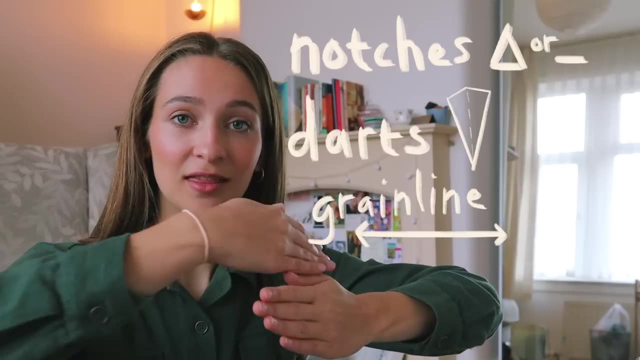 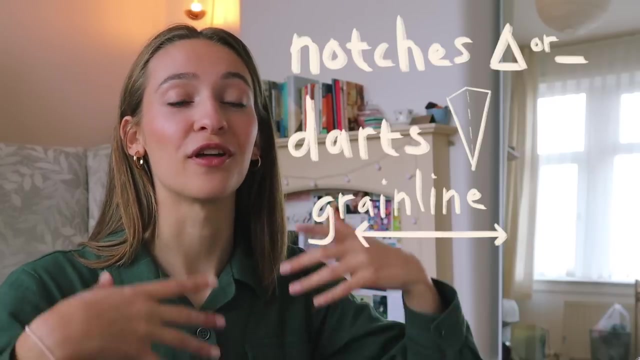 represents the direction in which the weave of your fabric should be going. So when you lay your pattern piece on top of your fabric, the weave of your fabric should be matching the direction of the grain line, if that makes sense. Basically, the purpose of a grain line is to help with the draping of a garment. They're 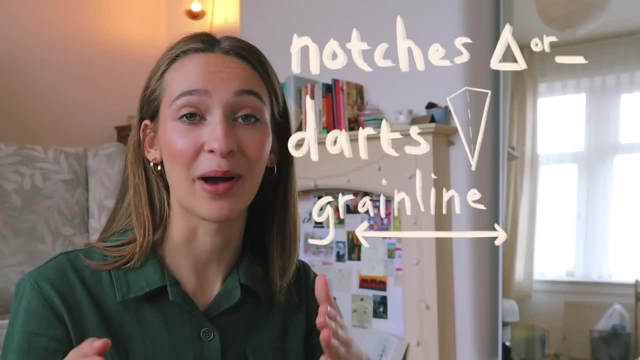 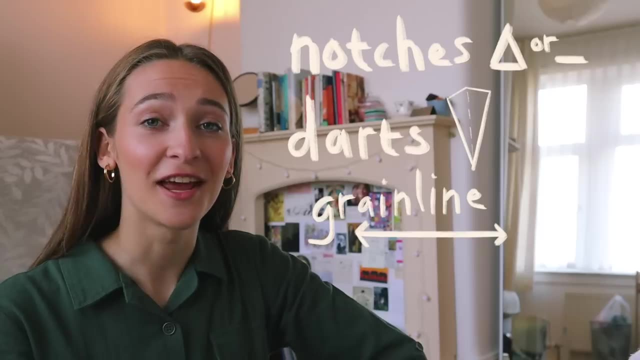 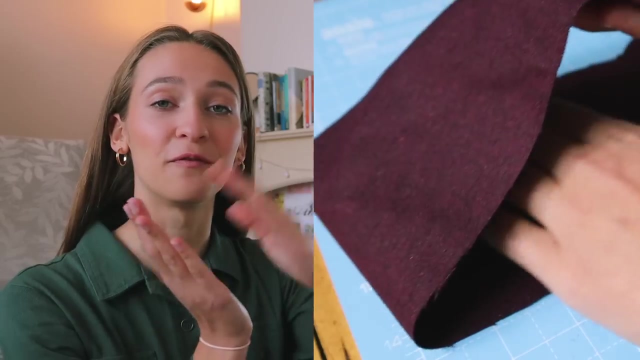 actually really important. and also, if your fabric has a pattern, a grain line makes sure that the pattern is going in the same direction on all the pieces. The next really common symbol is cut on the fold. This symbol simply directs you to fold your fabric over, align your pattern. 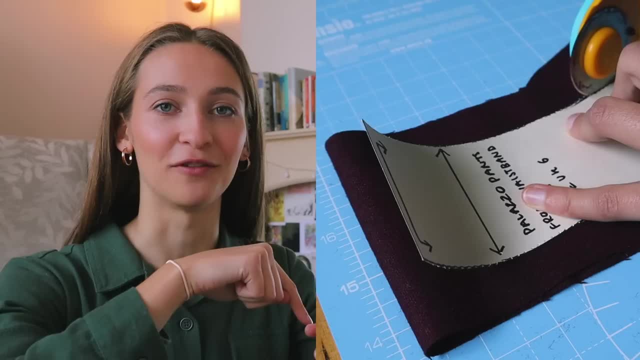 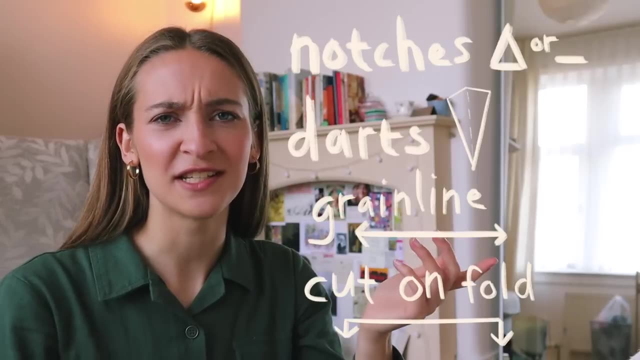 piece alongside the folded edge and then cut around it. That means you're you'll end up with a piece which is double the size and also perfectly symmetrical. You often see these cut on the fold symbols on like front waistbands or collars, things like that. Now, 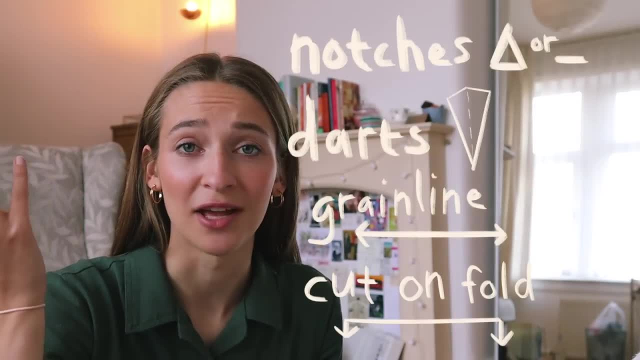 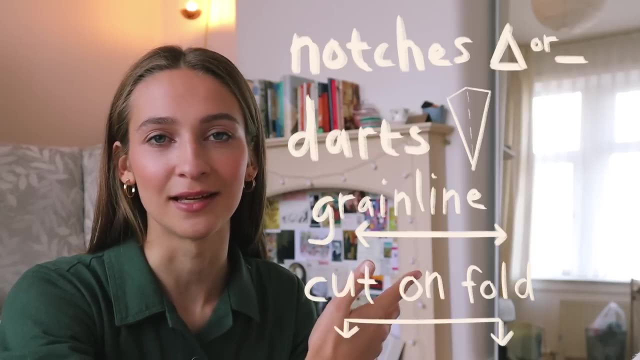 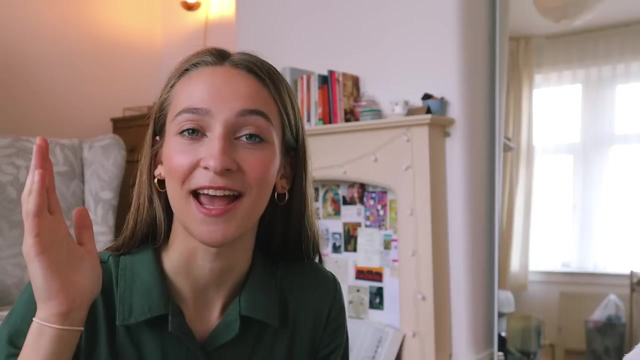 obviously, the more advanced and complex a sewing pattern is, the more symbols you might encounter, but for now these are the most common, the most basic, to get you started. So once you've traced your pattern and you understand all the symbols, it's time to cut out your fabric pieces. 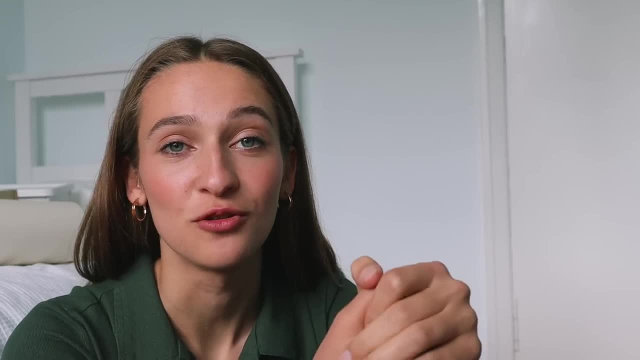 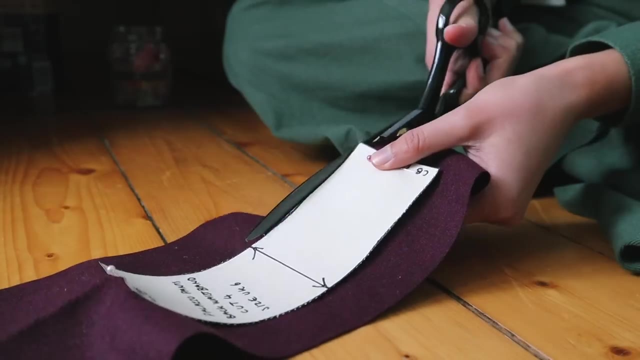 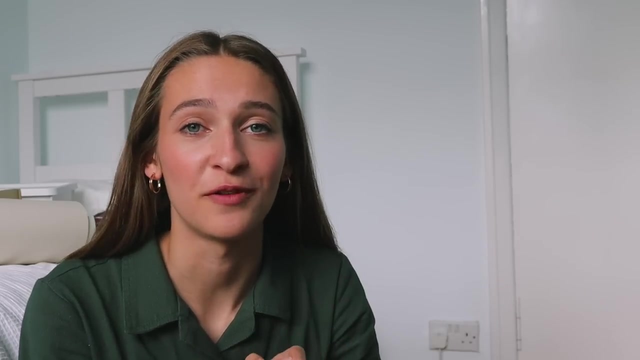 Okay, so there are a couple of different ways you can use to cut out fabric, One way being you can pin your pattern onto the fabric and then just cut around it with a pair of fabric scissors like these, Or you can lay your pattern flat on top of your fabric. use some random miscellaneous. 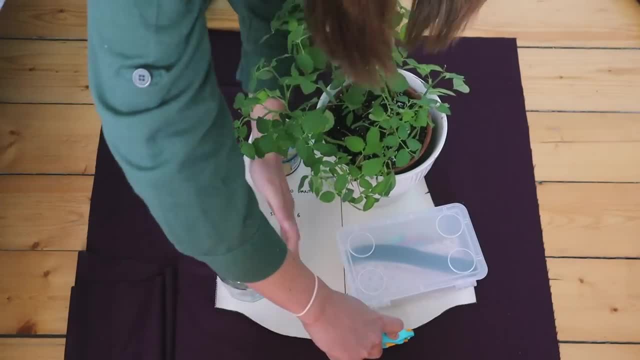 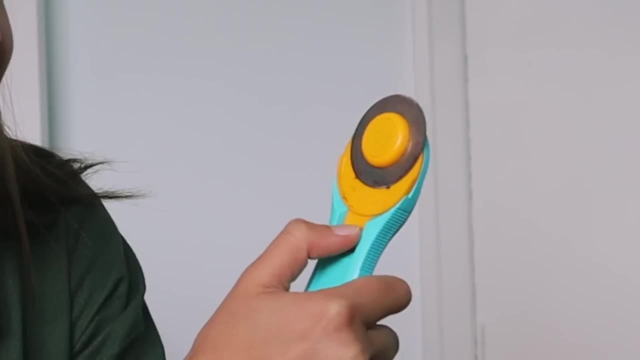 objects and then just cut around it with a pair of fabric scissors like these, Or you can use some random miscellaneous objects to weigh it down and then slice it using a rotary cutter, which is essentially just a pizza cutter, but for fabric. Usually, when you're cutting, you're 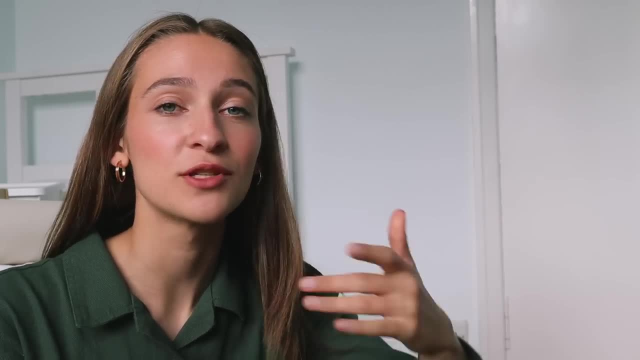 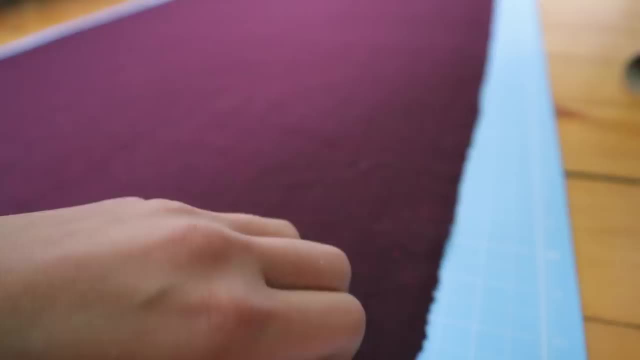 cutting two of the same thing, like two legs, two arms, two pockets, etc. etc. So to make the process a little bit quicker and easier, I recommend folding your fabric over so you're cutting through two layers at the same time and this makes sure that they are even and also 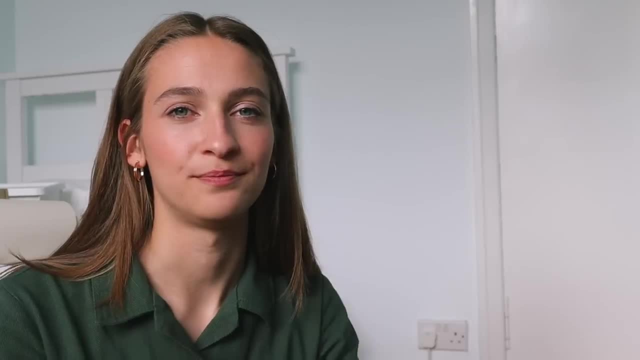 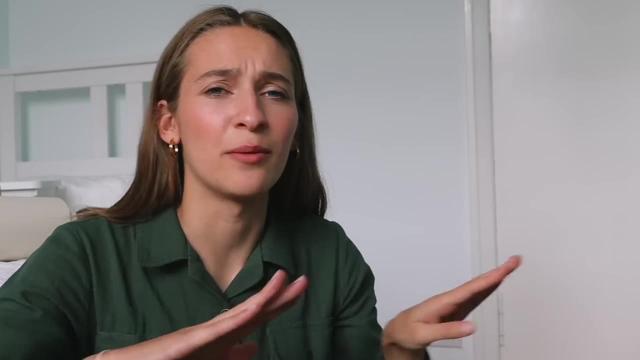 compact. So if you're cutting through two layers at the same time, you're cutting through two layers completely symmetrical, which is what you want. And, of course, when you're cutting, don't forget to follow the instructions on the pattern, Things like the grain line. make sure your fabric is in the 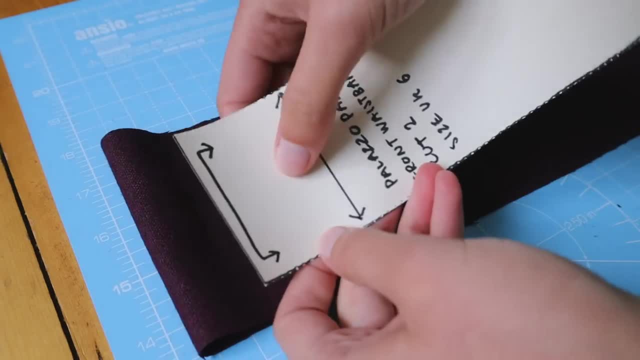 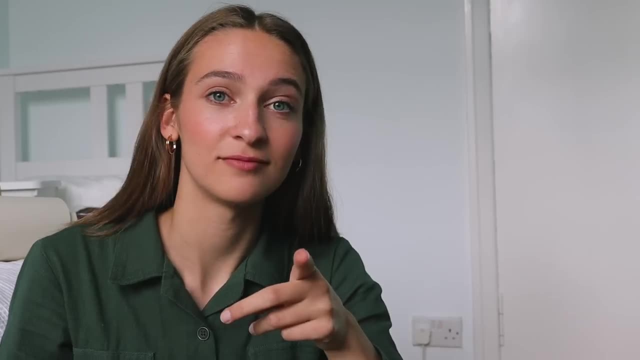 right position. Things like cutting on the folds if something needs to be double the size. Things like snipping in your notches- that's really easy to forget. Don't forget, And before you know it, you should have your army of fabric pieces ready to be assembled. 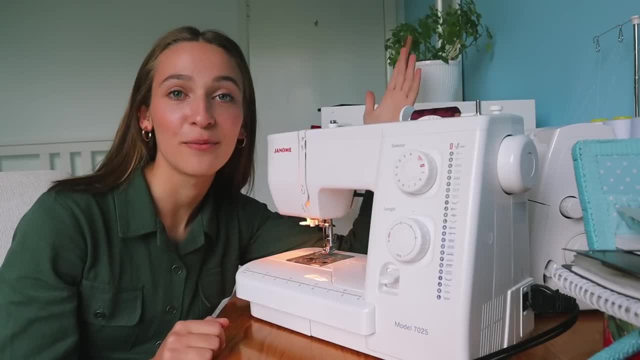 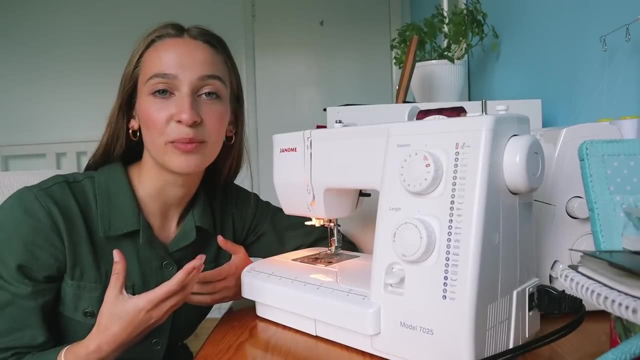 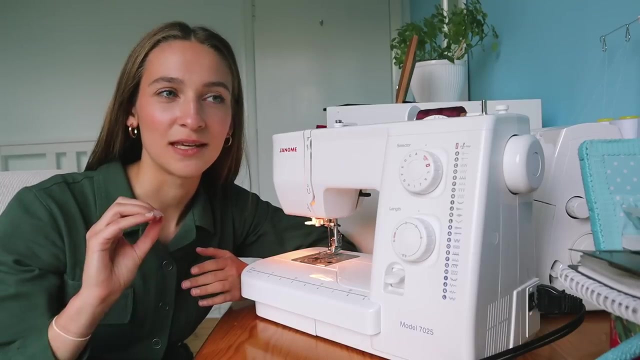 So you've traced your pattern, you've cut out your fabric. all that's left to do is: yeah, you still have to sew it. Usually, sewing patterns come with instructions, and the more beginner friendly a pattern is, the more comprehensive the instructions tend to be. So these are the instructions for my palazzo pants. 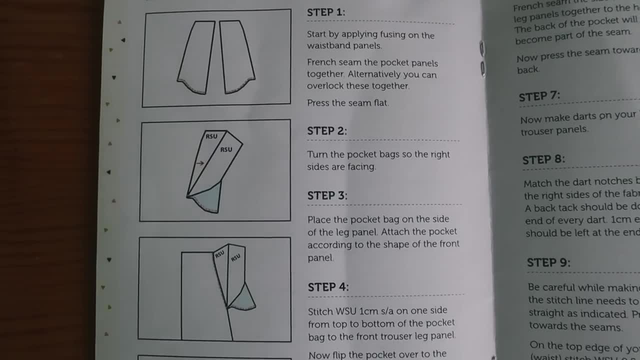 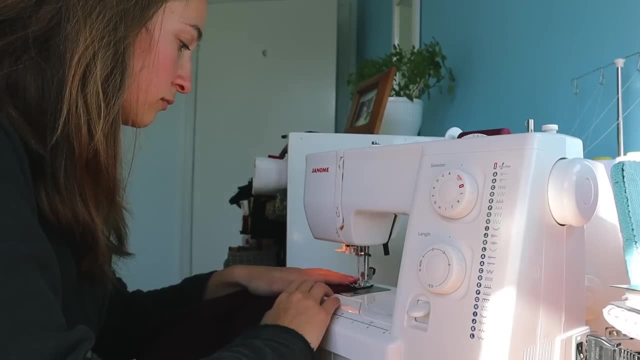 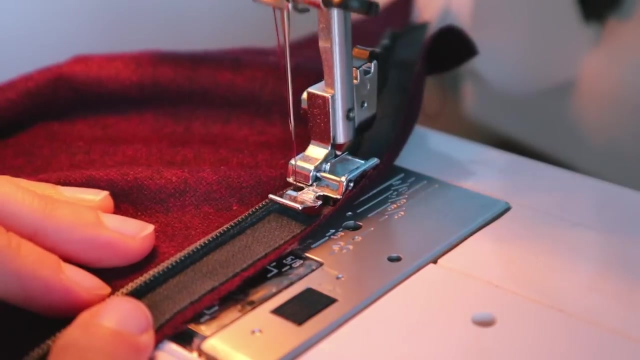 and it's been laid out in a really clear step-by-step format, which is how you'll find most pattern instructions. I'm not going to go into much detail about the palazzo pants, but basically follow the instructions step by step, take your time and just keep sewing until, hopefully, you reach something.